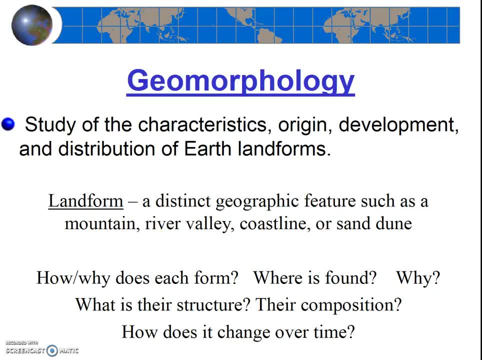 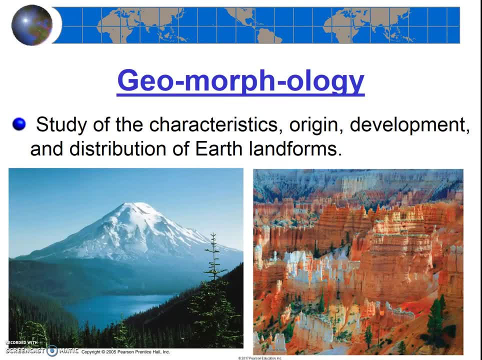 Pretty cool stuff really And it's pretty neat to be able to read the landscape like that. Take a few moments to look at the photos shown on this page. The one on the right is the opening photo from the chapter. If you didn't do so when you read the chapter, go back and read the seeing geographically questions at the beginning and end of the chapter. 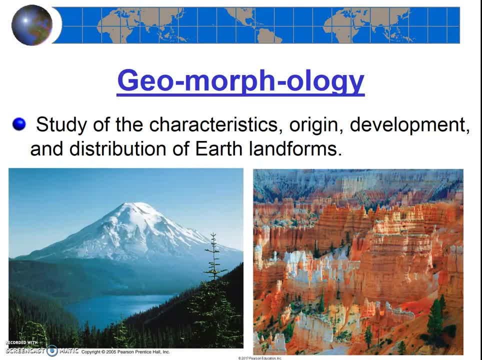 I encourage you to make a point of reading the seeing geographically questions in each chapter. Great photo: huh. What climate appears to exist in this region And why would you say that? How would you describe the rocks and the landforms, And what do you think caused some of these features that you see in this figure on the right? 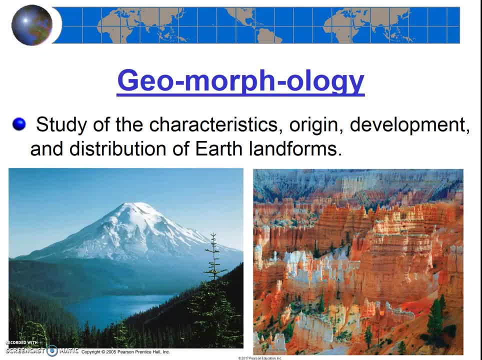 Based on your textbook reading, what type of rocks do you think are present in this photo? Why, Anyway, the American Southwest is a great place to study rocks and landforms because they're readily available for us to see them, And this picture here is in Bryce National Park in Utah. 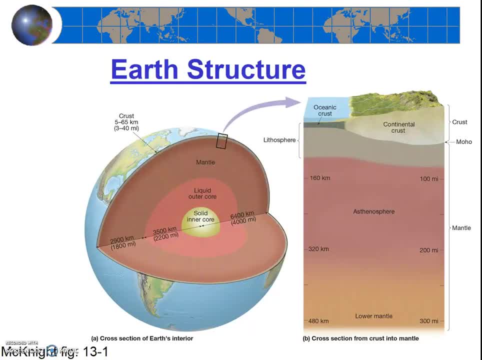 As we begin our study of Earth landforms, we first need to have a general understanding of the Earth's structure and composition. How was the Earth put together And what is it made out of? Well, first, the Earth has a layered structure. 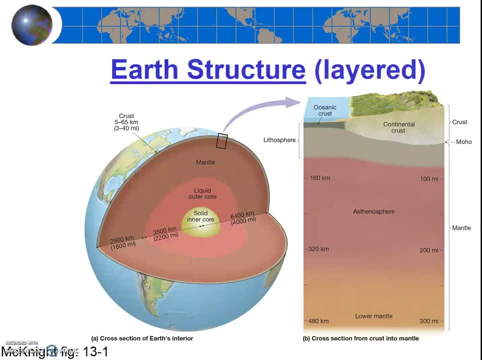 And, notably, there are two ways that we can discuss the layered structure of the Earth. We can identify the Earth's layers based on the composition of the layers, that is, what the rocks are made of. Or we can identify the layers based on the physical properties of the layers, how they act. 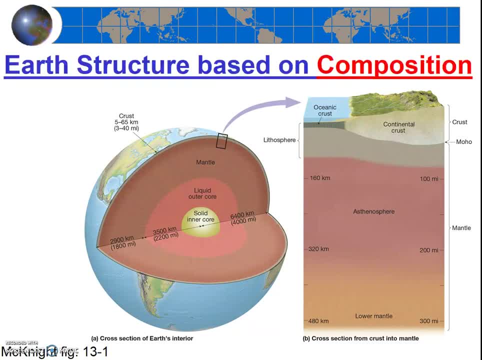 Great. First, we'll discuss the Earth's layers. based on composition, There are three layers, each made of a different material. The layers are called the crust, the mantle and the core. You should memorize these three terms and also memorize what they are made out of. 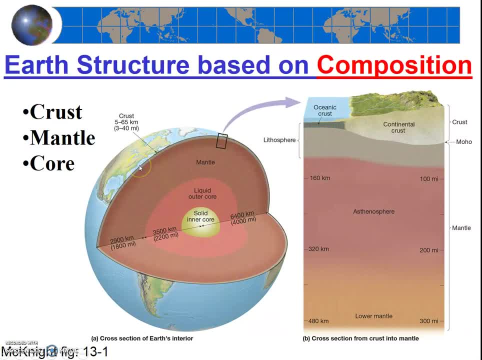 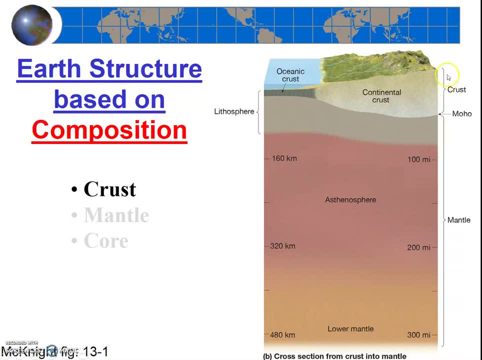 First we'll begin with the crust, the outer layer shown here as well. So this crust is the outer layer And obviously the Earth's crust is made out of many different rocks. Otherwise, rock identification in geology lab would be pretty easy right. 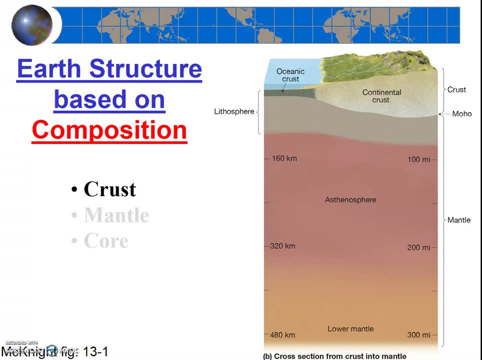 However, we can make some pretty good generalizations to try to simplify things a bit, In particular if we're looking at what the crust is composed of in the ocean. the ocean crust is made out of a rock called basalt, which is a dense black volcanic rock. 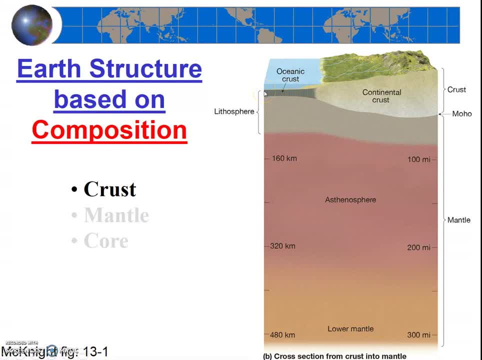 Other things to note about the oceanic crust is: it's only about five miles thick, which is very thin compared to the 7,900-mile diameter of the Earth. So this basalt contains a lot of iron and it's quite dense. 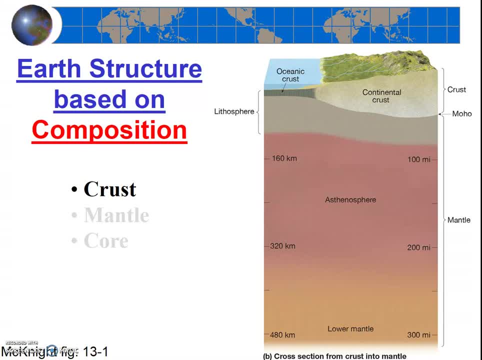 roughly about three grams per centimeter cubed. On the continent there's different rocks that dominate And of course the continental crust. the continental crust is really composed of many different rocks But overall the composition approximates granite. So we say the continental crust is composed of granite. 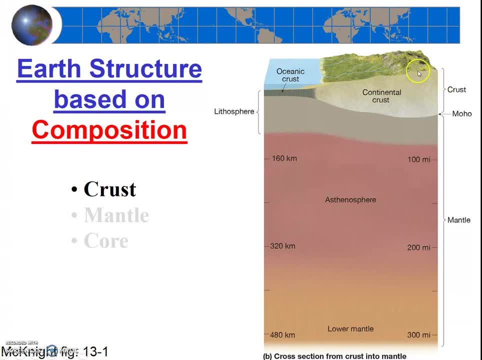 Another thing you can see on this diagram is that the continental crust is much thicker than the oceanic crust. On average, it's about 25 miles thick, And this granite that makes up the continental crust is much less dense than the oceanic crust. 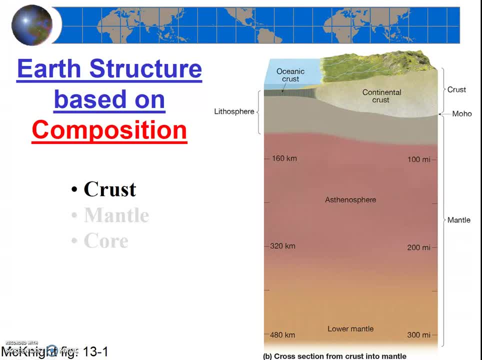 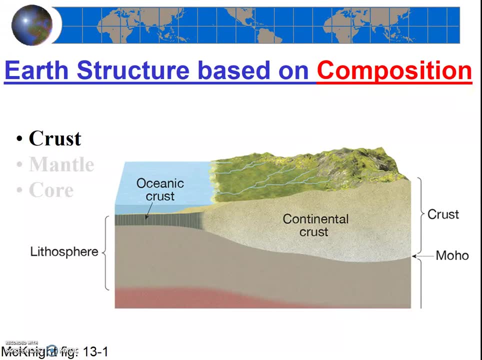 The density is about 2.7 grams per centimeter cubed. All right, So if you were asked what the composition of the Earth's crust was, you should ask me which part of the crust- The oceanic crust- is made out of basalt. 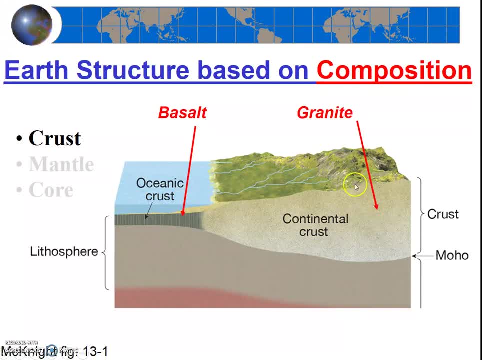 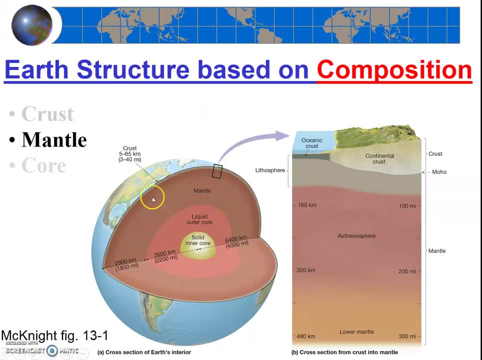 and the continental crust is made out of granitic material- granite. Next, we'll move deeper into the Earth and we're in the layer called the mantle. The mantle makes up the greatest percentage of the Earth in terms of the three layers. 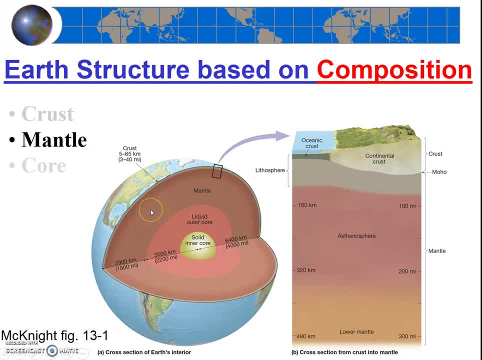 And over 80% of the Earth by volume would be considered mantle material. The mantle is about 1,800 miles thick and it's primarily composed of a rock called peridotite. Peridotite is also very iron-rich, and the density of peridotite is actually greater than basalt. 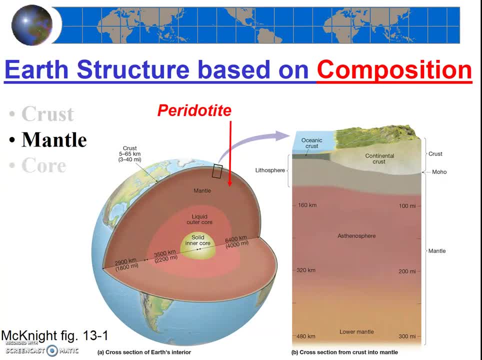 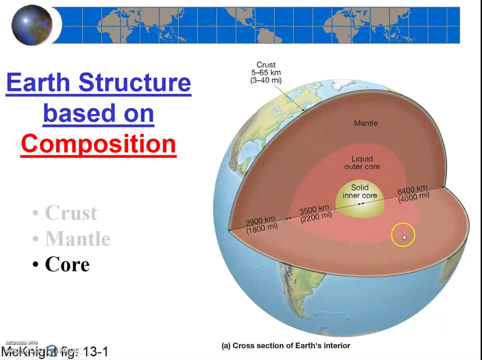 It's 3.3 grams per centimeter cubed. Moving deeper in, we now are in the core. The core is the third layer, the inner layer of our three layers, and it's at the center of the Earth. There are two parts to the core: the outer core and the inner core. 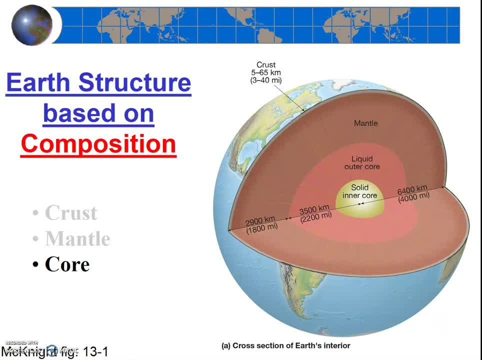 but for now we'll treat them together because they're both made up primarily of iron and nickel. The core is about 2,200 miles thick and, as you can imagine, if it's made up primarily of these metals, it's very dense, at about 11 grams per centimeter cubed. 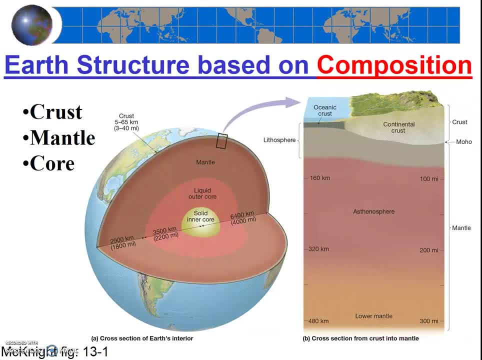 So, in summary, if we're talking about the layers of the Earth based on the composition of the layers, we have three layers: the crust, the mantle and the core. The crust is made out of basalt in the oceans, granitic rock on the continents. 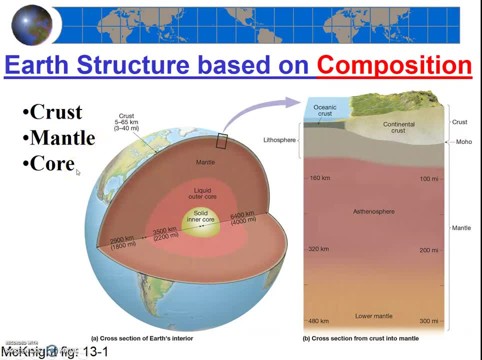 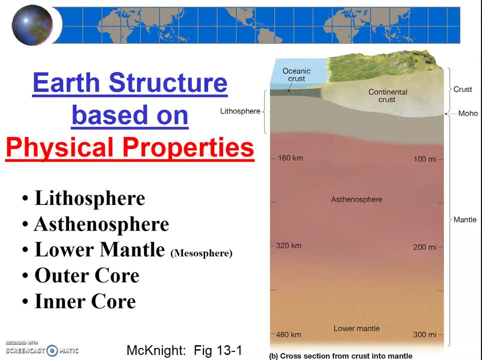 the mantle is made out of peridotite and the core is made out of iron and nickel, primarily. Next, let's discuss the Earth's layers, based on how the different layers act, their physical properties. There are five layers. if we focus on the physical properties of the layers, 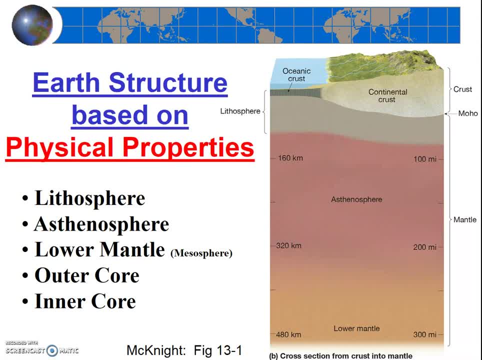 For physical properties. for our purposes, we're going to be primarily interested in whether the layer is solid or not solid. So there's five layers based on physical properties: The lithosphere, the asthenosphere, the lower mantle, which some textbooks call the mesosphere. 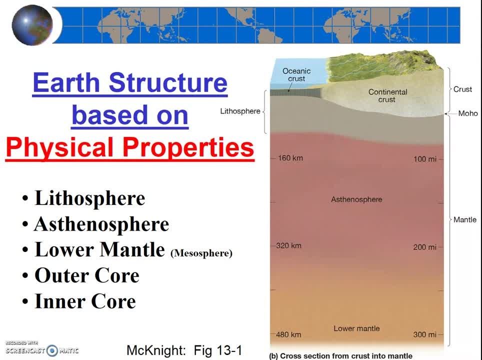 the outer core and the inner core. On this diagram you can see that only three of the layers are shown: the lithosphere, the asthenosphere and the lower mantle. But on the other future diagrams we'll see the outer and inner core as well. 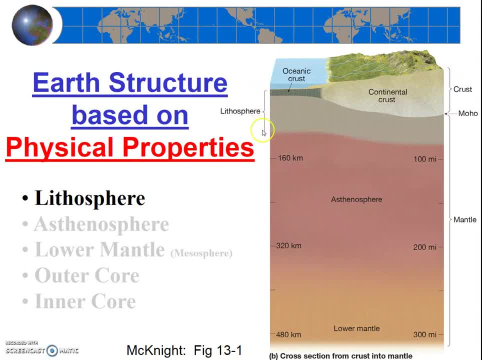 So first let's consider the outer layer, the lithosphere. In terms of its physical properties, the lithosphere behaves as a solid, rigid rock, And you knew this. You don't see pools of magma when you go hiking. The prefix lith means rock. 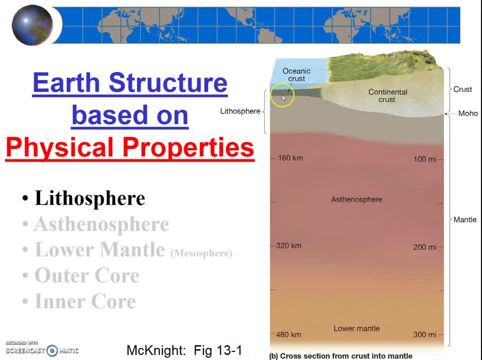 And notice here that the lithosphere contains all of the crust and the top of the mantle. That's very important. It's not just crustal material, It's the crust and the top of the mantle. Also importantly, the lithosphere is what makes up the plates of plate tectonics. 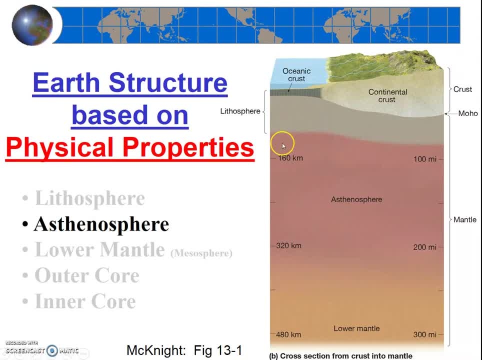 which we're going to discuss next week. The next layer down is called the asthenosphere. This is all mantle material, so it's peridotite, But the rocks of the asthenosphere are much weaker than the rocks of the lithosphere. 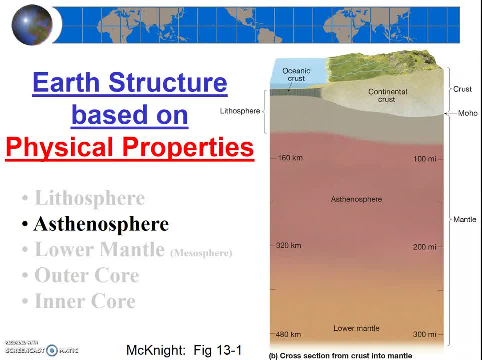 Indeed, astheno is a Greek root which means without strength or weak. This layer is not all liquid, but there are pockets of magma and in general, the rocks are much more easily deformed than rocks in the lithosphere. 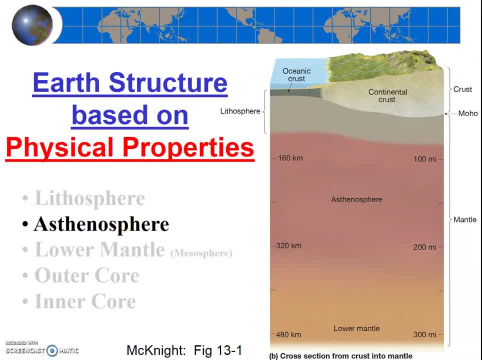 Think of clay or thick solid tar. Why are these rocks in the asthenosphere so weak? Well, as you go deeper in the earth, the high temperatures deep in the earth are the primary reason. Remember again, this is mantle material. 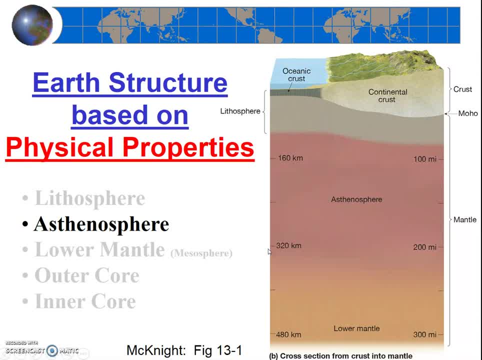 so the asthenosphere is a layer of mainly solid but quite easily deformed peridotite, this weak layer, with some pockets of magma. Moving deeper down we have the lower mantle. Some books call this layer the mesosphere, which I liked because meso means middle. 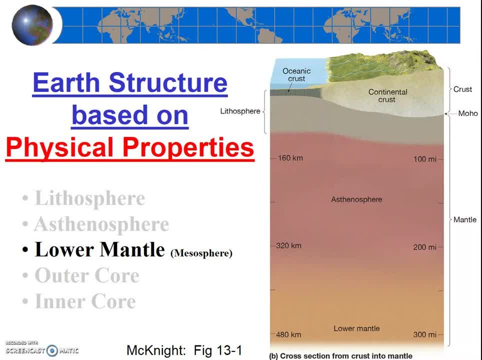 and it's right in the middle of these five layers, But it can be a bit confusing because you remember that the atmosphere also has a layer called the mesosphere. Anyway, the lower mantle, or mesosphere, is solid. These rocks are much stronger than the asthenosphere. 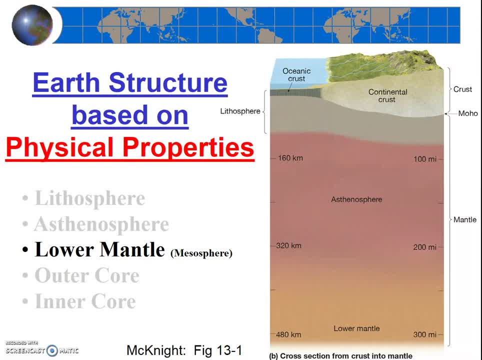 even though it's still mantle material. it's all peridotite. So why are the rocks solid in the lower mantle? It's crazy hot down there. It's certainly easily hot enough to melt the rocks. What's keeping them solid? The answer is pressure. 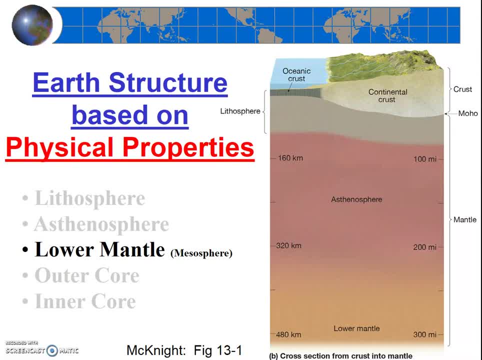 The deeper you go down into the earth, the higher the temperatures, but also pressure is increasing dramatically. The pressure is essentially pressing the atoms into their denser, solid arrangement rather than the less dense flowing liquid. Just as you can compress a gas to make a liquid. 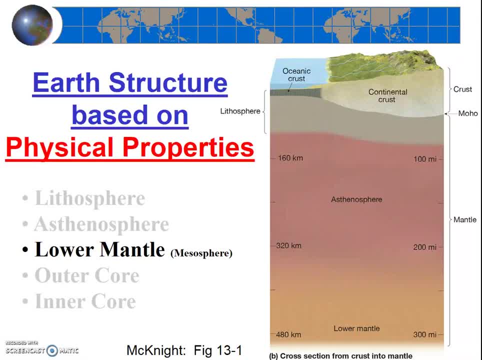 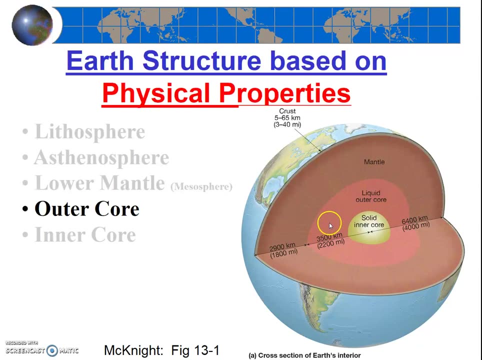 you can also compress a liquid to make a solid. So the rocks in the lower mantle are certainly hot enough to melt, we would think, and they would certainly melt at that temperature on earth, but the intense pressure keeps them solid. Going deeper still, we get to the outer core.